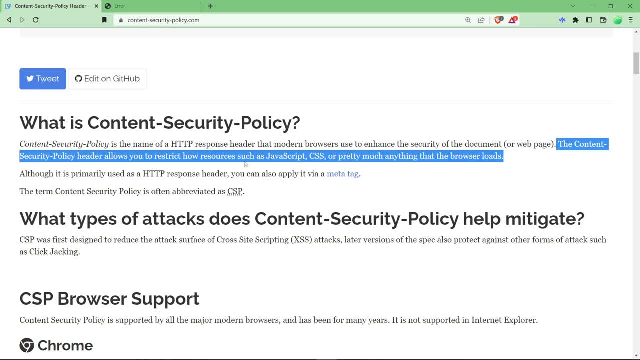 okay, as you can see, here i have highlighted a text. uh, it basically says that it is used to restrict how resources such as javascript, css or pretty many things that are browser loads. okay, it basically means that it is used to restrict the things with the browser loads. okay, you can. 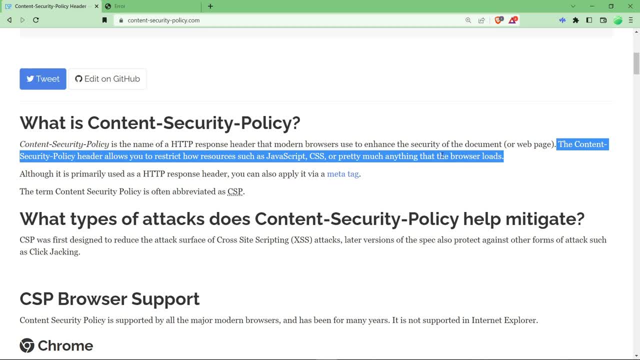 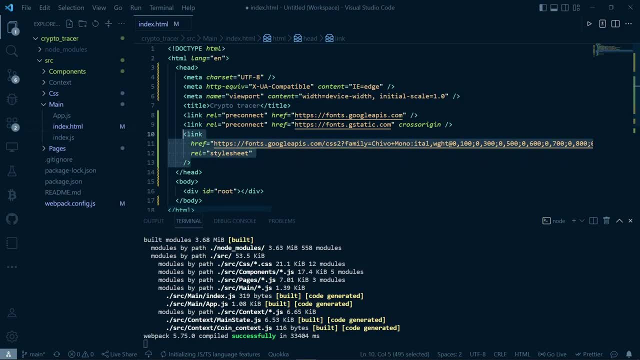 use uh for restricting the uh any links to load it uh in your web app. okay, uh, this basically means that it is used to restrict the things with the browser loads. okay, you can use. basically restricts this uh link in my app to load in my app. okay, what it means is this not? and this: 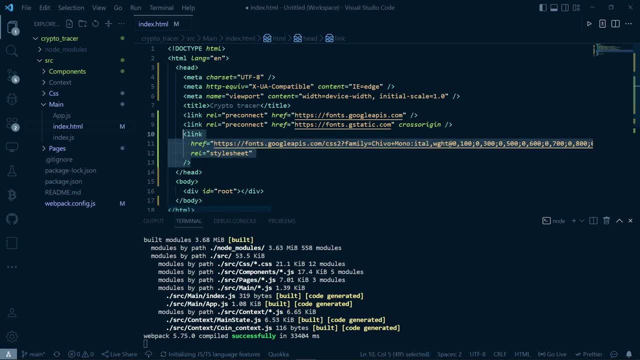 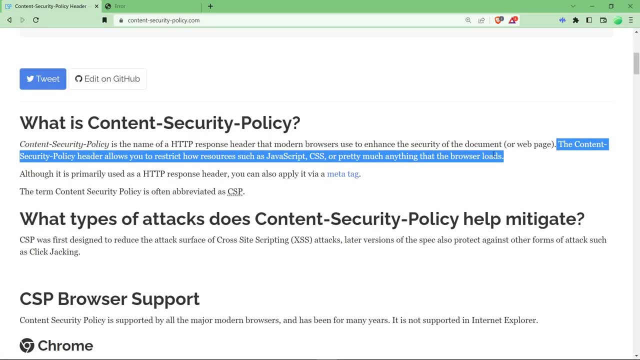 is not allowing me to load this link in our web app. okay, to solve this error, you just have to navigate a little down. okay, uh, you can even secure your web app by using this. they will just have to add a meta tag, uh, specifying that which url that you can load in your 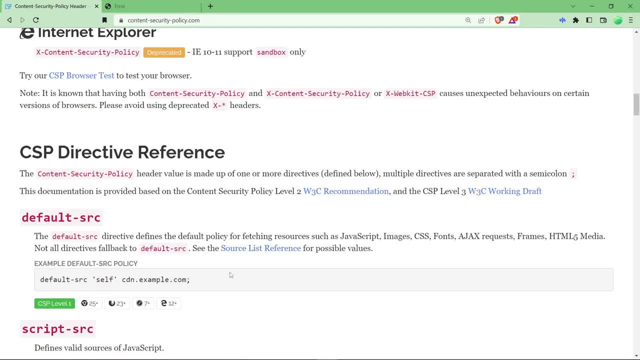 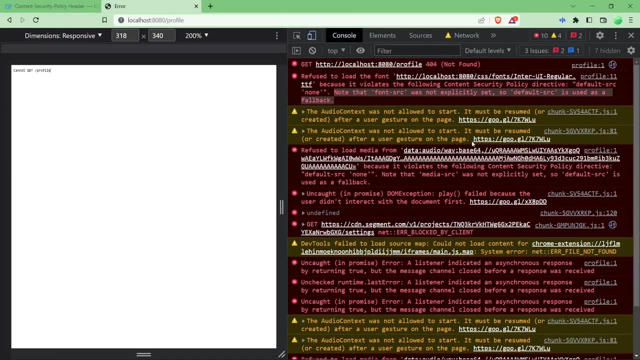 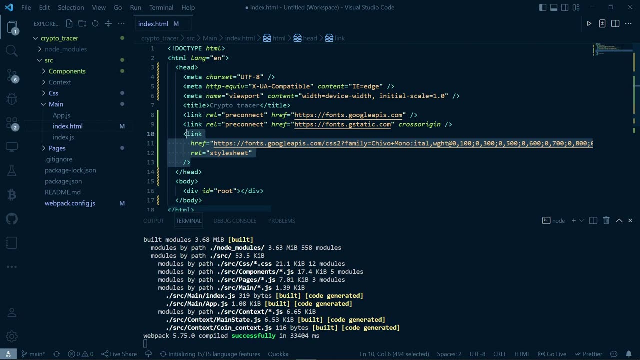 web app. okay, if you go a little down, uh, and script src and style src. okay, let's see what's the error which you are wanting. we are getting that. the font is actually okay because of fonts. we are getting this error and this is our link here. if we add another line, okay, this one, uh, let 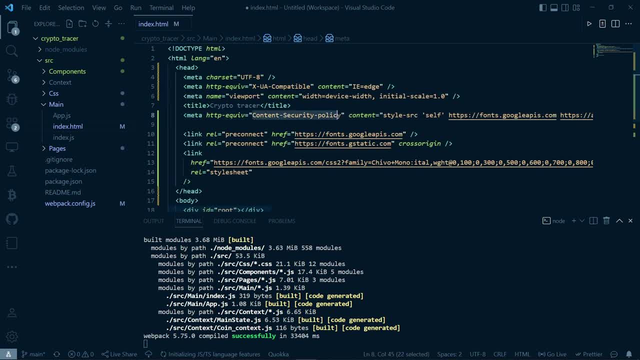 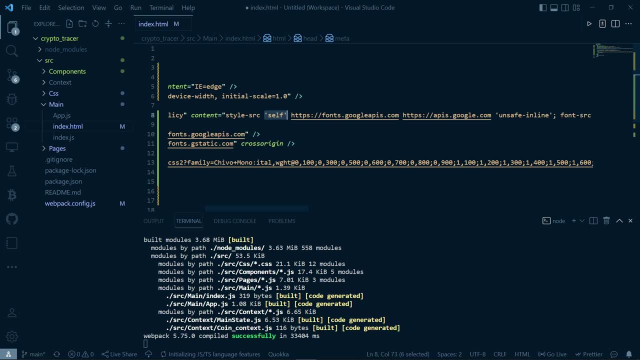 me explain this. this is a meta tag having content security policy, which basically says that the style src means: uh, the style sheet can be either a self or it can load from this url or from this url. okay, uh, and this another one is font src. this is for style sheet and, as you can see here, 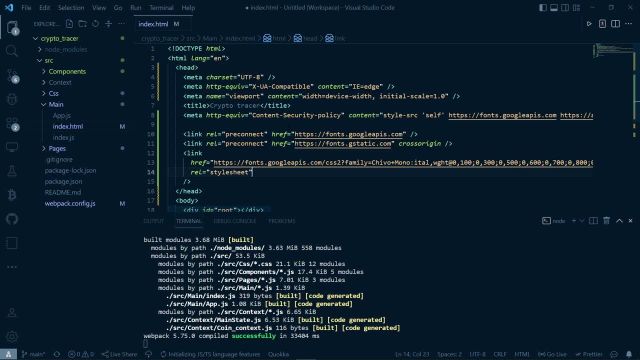 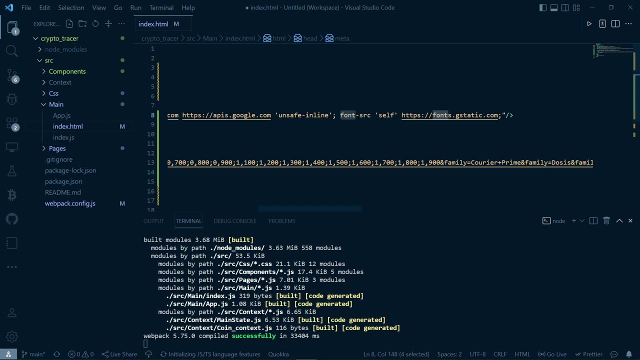 this is a style sheet. okay, fonts are loading from style sheet and another is font src. if you have another external fonts that want to load in your app, you can have this kind of thing: font src self and the link which you have which you are loading from. okay, uh, it could be not only a one link, okay. 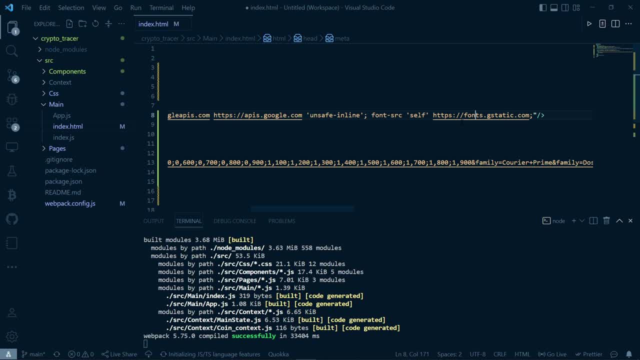 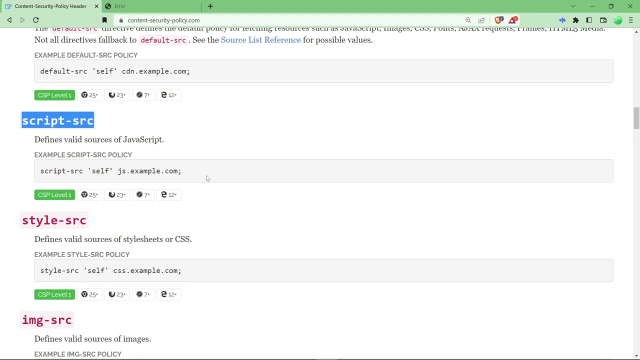 you can have multiple links, either fonts or anything else. okay, if you want to load a javascript uh kind of thing like jquery, you have to add cryptos, as you see. here it is the uh. it is written here: defines valid sources of java javascript. okay, you just have to copy this. 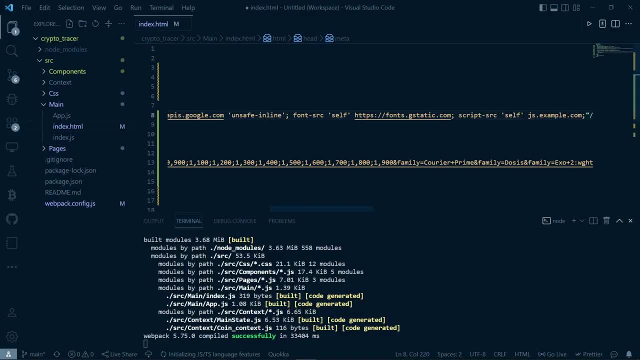 and you just have to paste it here, okay, in this meta tag, and here you have to replace this link with the link which you are loading javascript from. okay, this basically means that, uh, javascript can be either a cell or and the link which you have provided. it can take it from there. 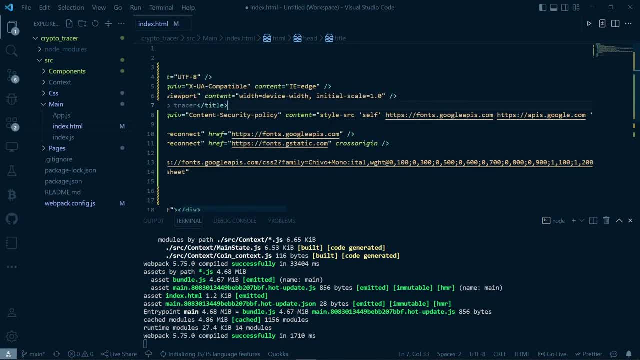 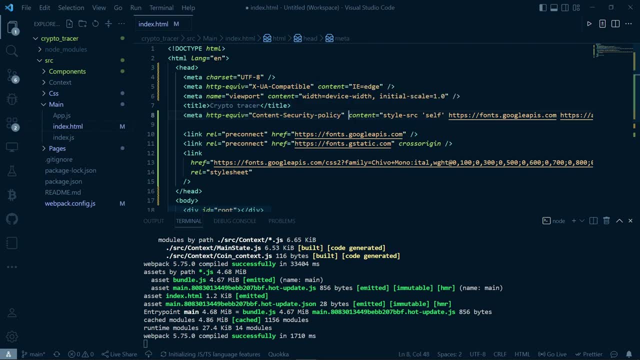 let us see if our error gets solved after adding this meta tag in our html document. okay, this error basically comes when you are using uh, webpack and all uh, and you can even use it for html if you are getting the error, view and angular and whatever. you are using security policies for all, okay, it's not uh for single one, okay, and 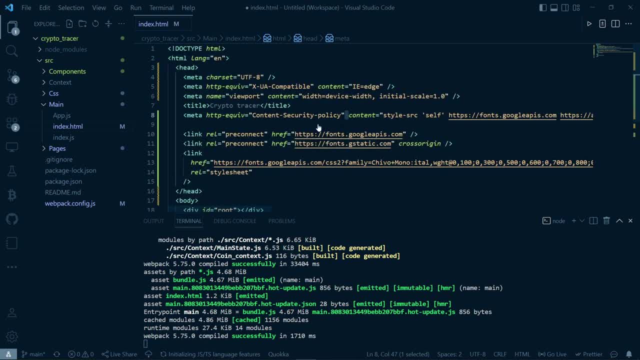 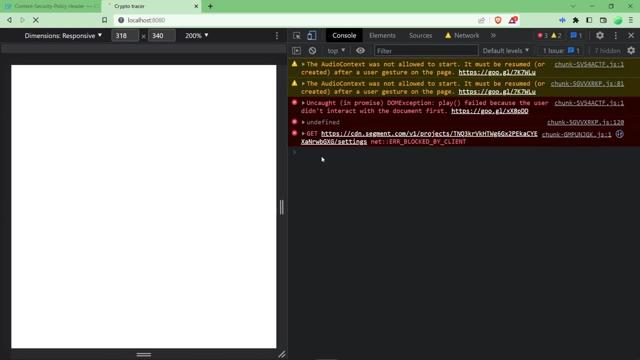 you are. you're in the react, it is automatically handled, and here in the back it's not automatically handled, so we have to add it manually. okay, let us see if our error gets solved or not, and if we refresh the page, we end up having this error. and okay, these are some other errors. 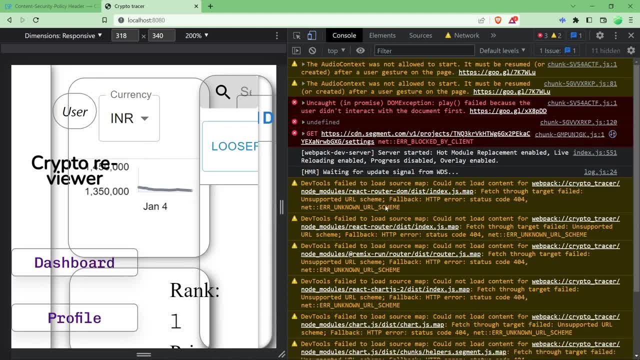 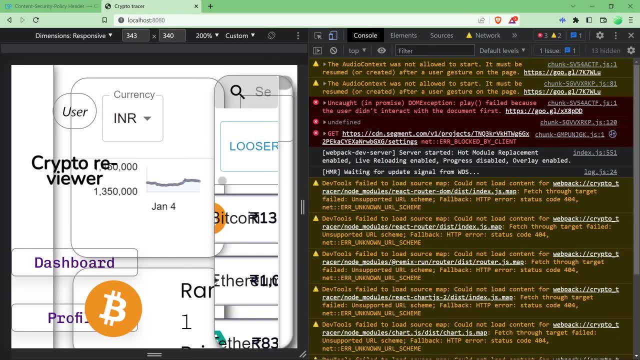 okay, this loading, as you can see here. uh, this is a website, okay, uh, it's fully loaded here. you can see there is no error from the content security policy. this is, uh, just app which is not responsive at all. okay, uh, don't mind this and this is how you can solve this. uh, if you are getting anything, 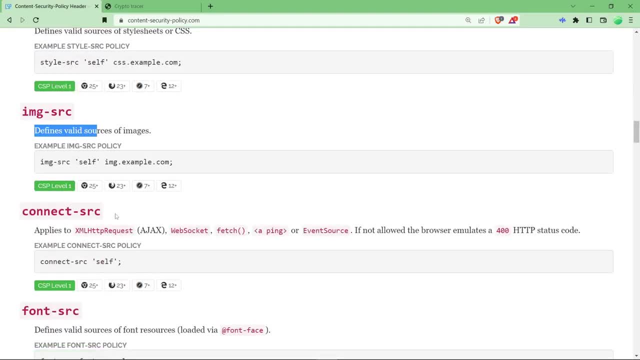 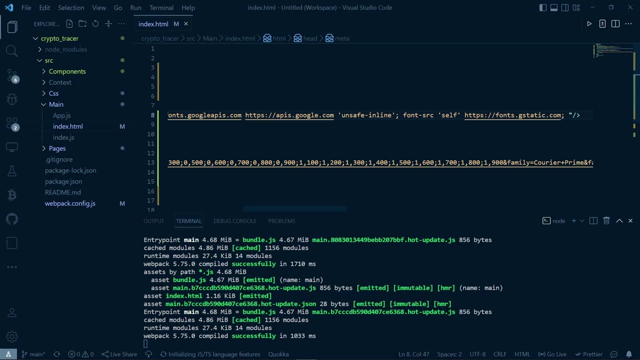 else, like, such as you may get uh image src error and contentront uh src error and you just have to add it here, like you just have to compete and you just have to add it at end and specifying the link which you are loading from. okay, and this is how you can solve it, this code. 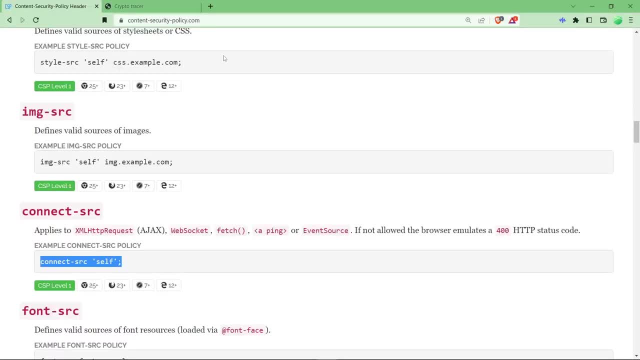 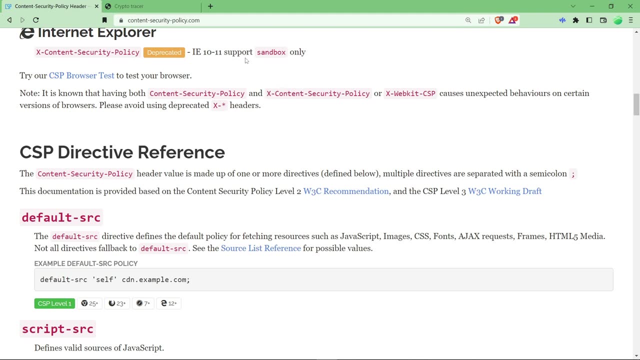 will be pinned in the comment section and the link for this website will also be pinned in the comment section. okay, thank you for watching this video and if you have any queries related to this or your error didn't got solved, uh, let me know in the comment section. uh, you'll get a solution for. 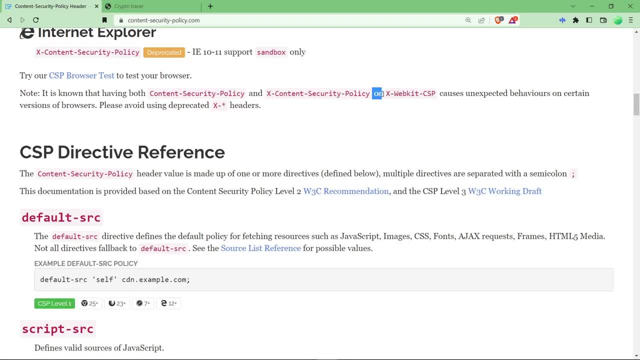 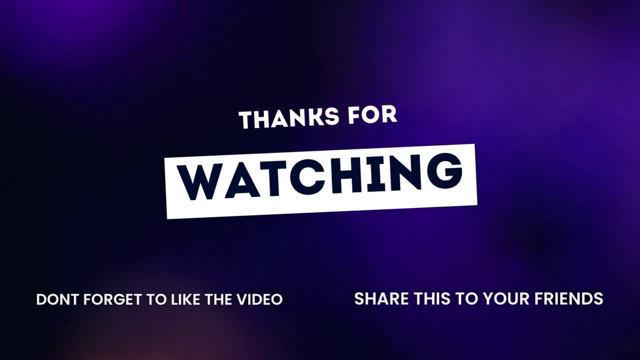 that within 24 hours and if the video was helpful, make sure to like this video and subscribe to our channel. thank you all.